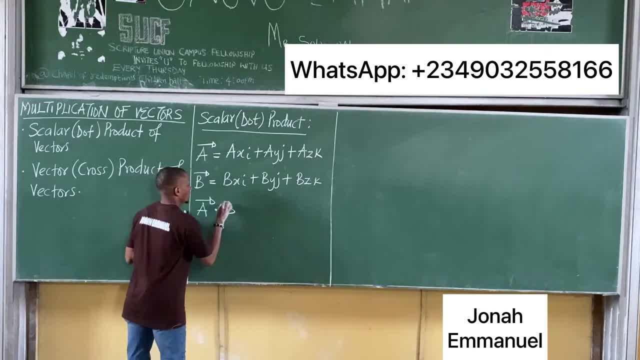 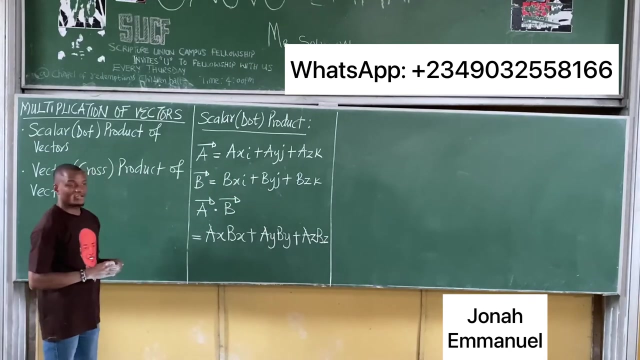 a dot b. So this is the dot product of this vector And mathematically, a dot b is simply equal to a x, b, x plus a, y, b, y plus a, z, b, z. So this is it. This is the dot product of the vectors. 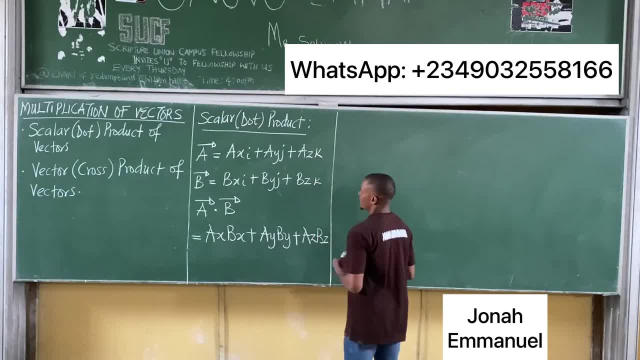 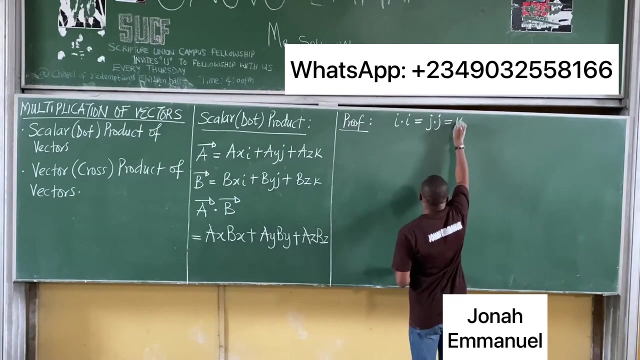 We look at the proof of this. Let's prove this. So proof, Let's prove this formula. To prove this formula, there's something you need to know, And that's the fact that i- dot i is equal to j, dot j is equal to k. 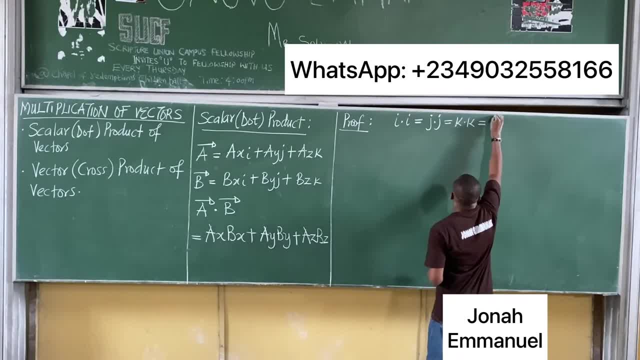 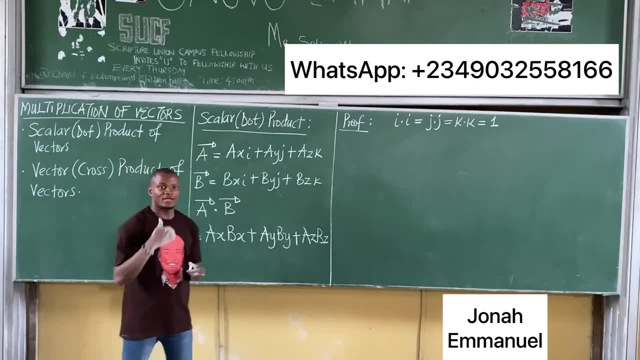 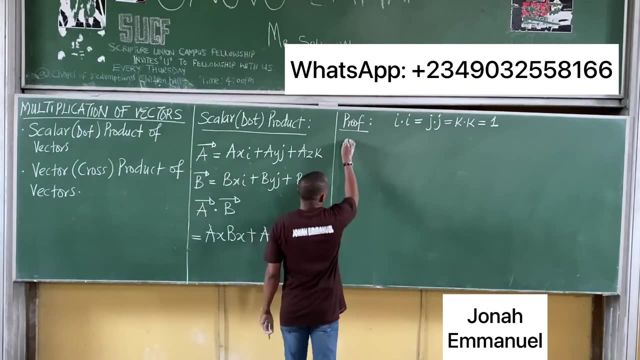 dot k, and that's equal to 1.. This is the identity you need in proving this formula: That i dot i equal to d dot j equal to k, dot k, and that's equal to 1.. Alright, so let's prove this. Let's see a dot b. 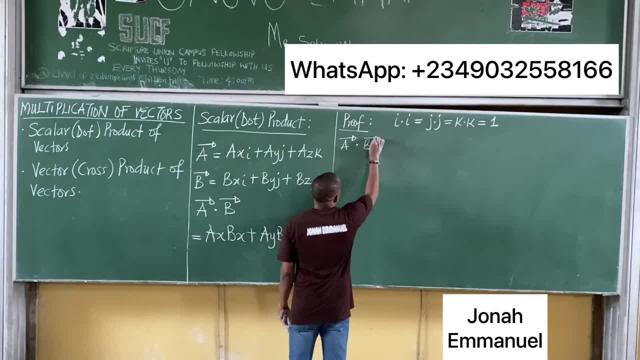 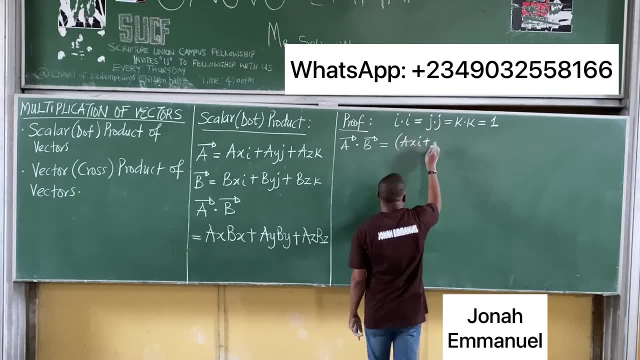 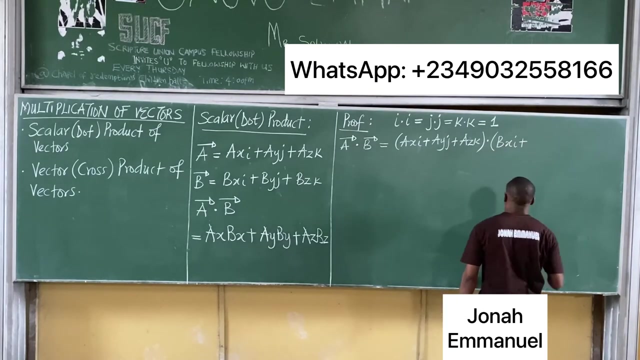 So in a more complex sense, a dot b will equal to a x i plus a 1 j plus a g k dot b, x i plus b, y j plus b z k. Now we said: i dot i equal to j dot, j equal to k dot k. 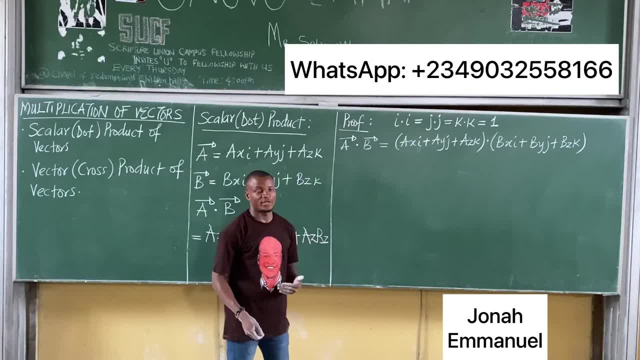 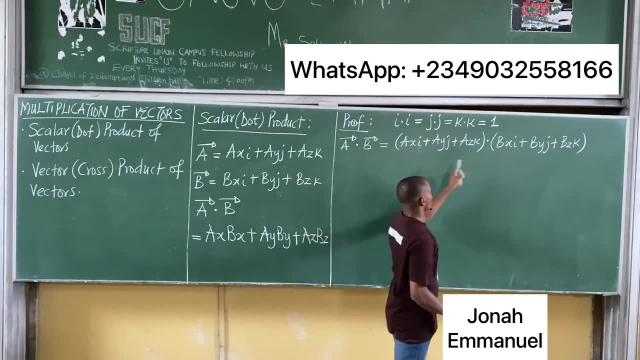 equal to 1.. All other thing is equal to 0.. All other thing equals 0.. So if I choose to multiply this, I'm having use everything here to multiply this. So I'm having a x times b x. so first of all, 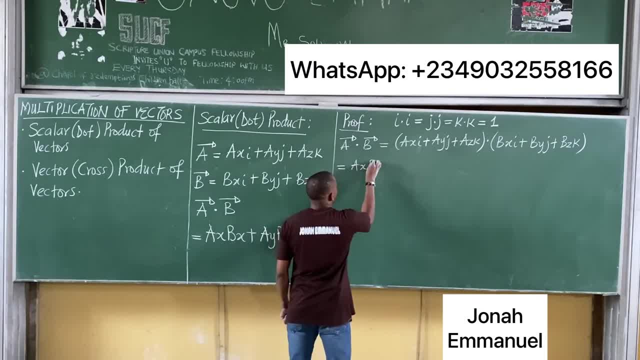 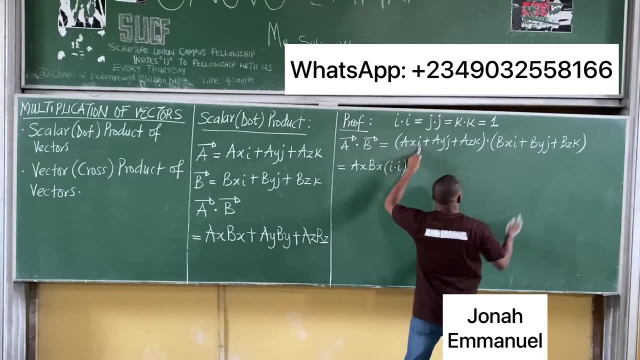 this is equal to a x b x and then to i dot i. so this is i dot i plus a x, i plus a x dot i. multiply b? y into h? g. a x b y, so a x b y. i dot j, so i dot j. 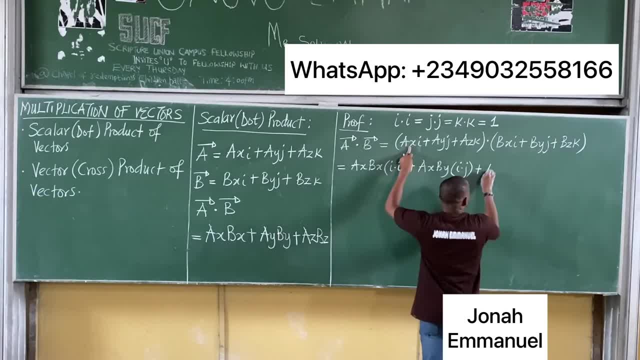 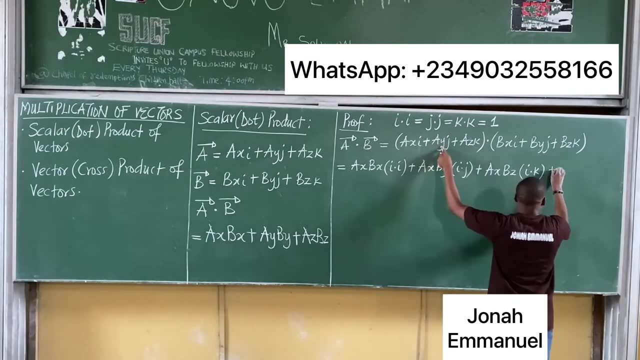 plus a x b z. so a x b z into i dot k. so i dot k. I'm not with a x come to a y, so plus I'm having a y b x, a y b x into j dot i, j dot i a y b y. 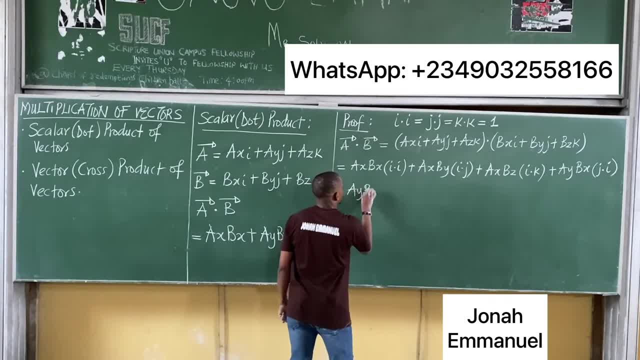 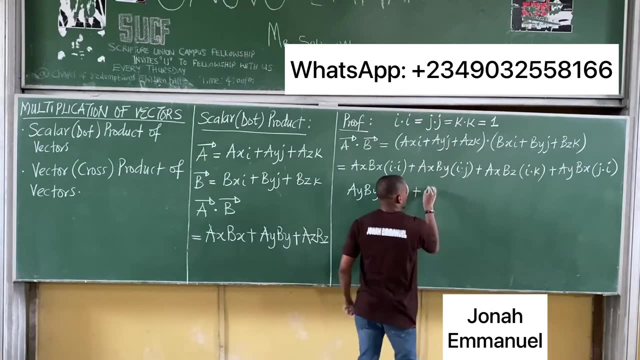 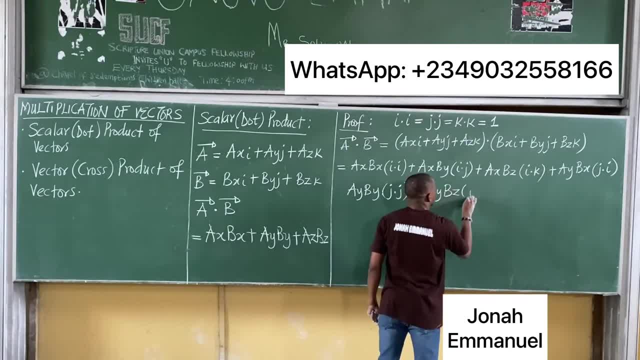 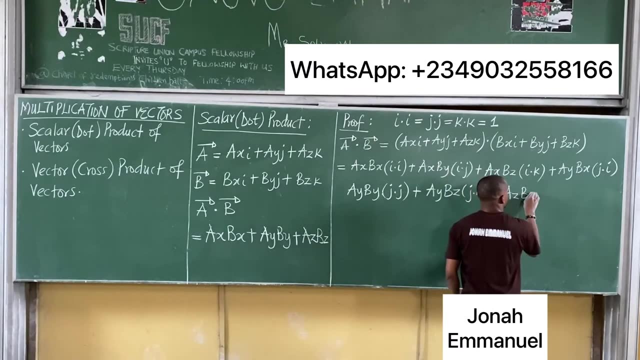 a y b z j dot k, so a y b z j dot k, so a y b z j dot k. so finally, I have plus a z a z a z b x, so a z b x. I have k dot i, k dot i, plus I have. 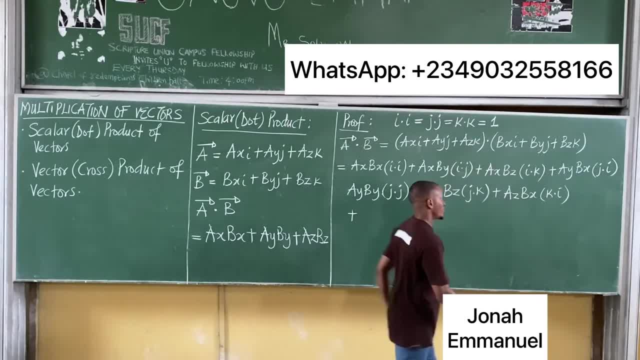 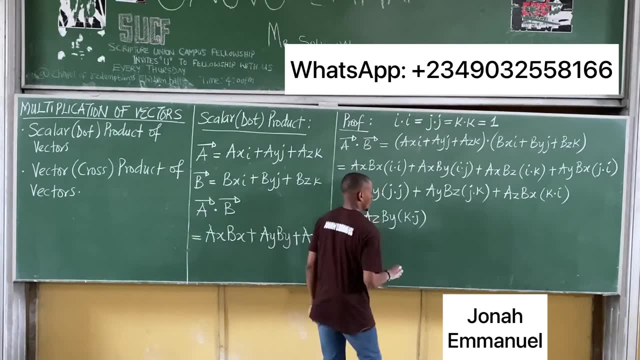 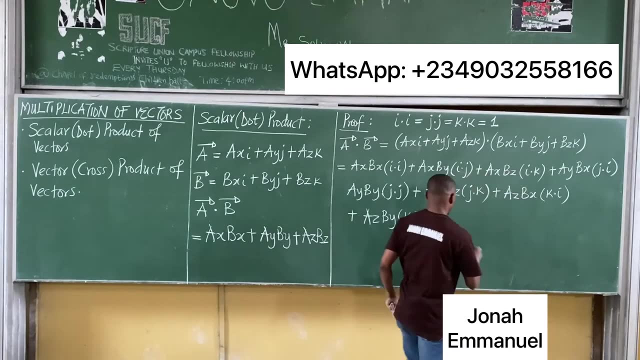 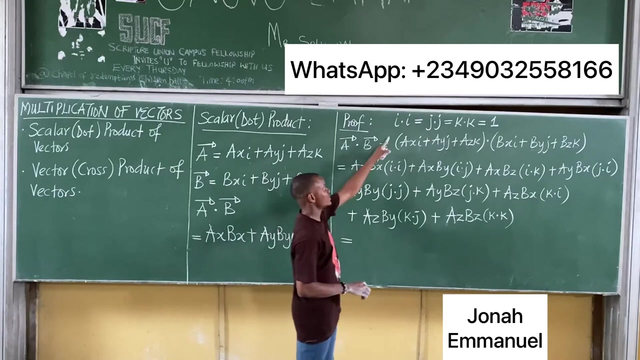 a z b y k dot j, a z b y k dot j, plus finally a z b z K dot K. so A C B C K dot K. Alright, let's bring in our condition. If you bring in our condition, we said I dot, I is equal to 1. 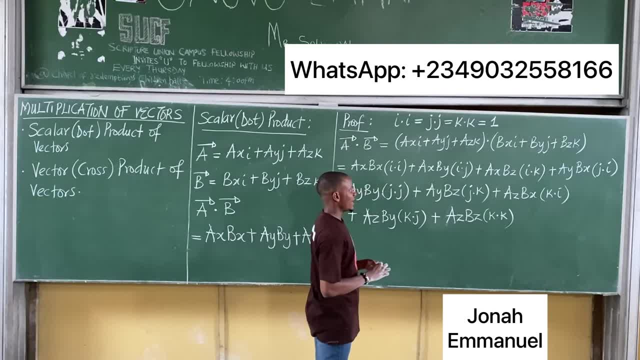 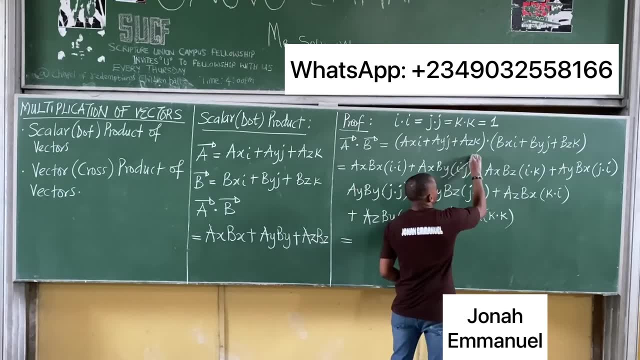 so this gives you 1. so automatically it's not I dot I or J dot J or K dot K, it becomes automatically 0. for instance, this one here gives you 0, this one here gives you 0, this one here gives you 0. 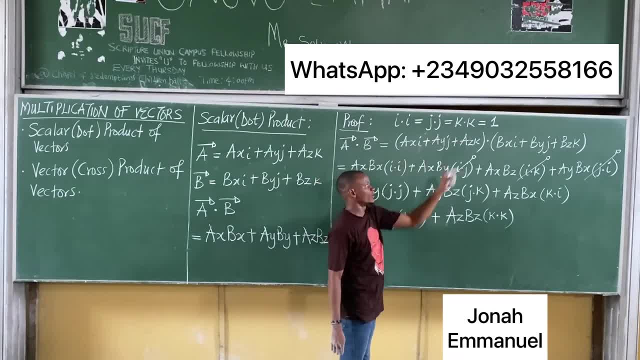 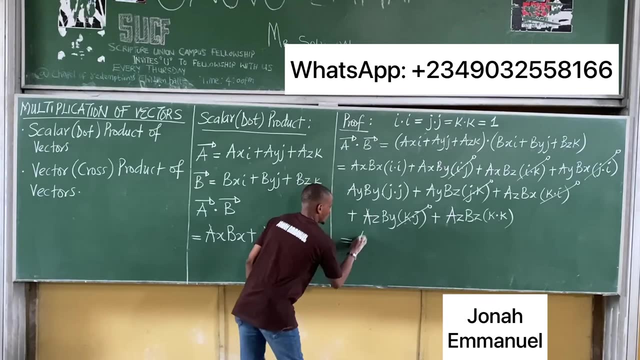 this is J dot J, which we said is equal to 1, so it stays. this one gives you 0, this one gives 0. this one here gives 0 K dot. K, we said is equal to 1, so I'm having this. so let's start with box. 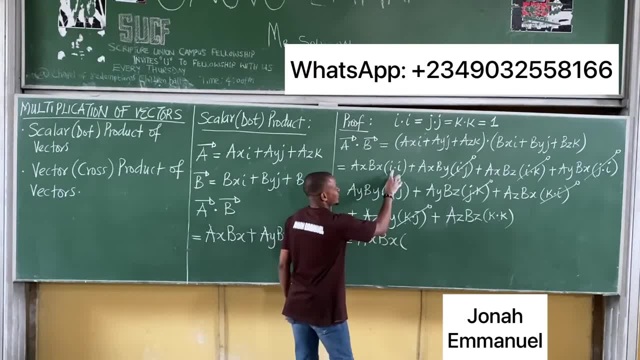 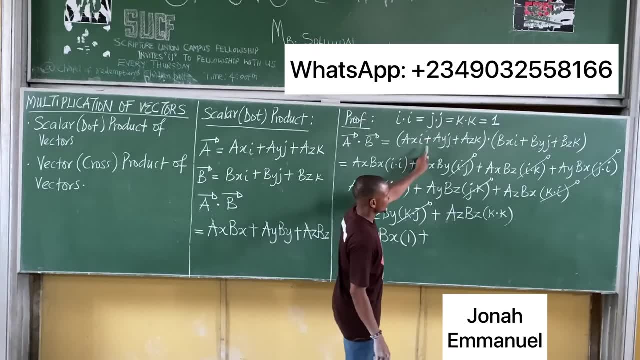 A, X, B, X into I dot I, which is 1 plus. so this one is 0, it's off. this is 0, it's off. this is 0. so this time 0 is 0, it's off. so plus A, Y, B Y. 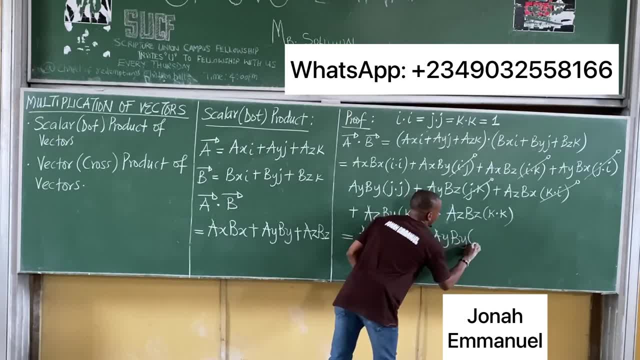 so A Y, B, Y times: 1 J dot J, which we said is equal to 1 plus this is this time 0, 0 is off. this time 0, 0 is off. this time 0, 0 is off. find that you have A Z, B Z. 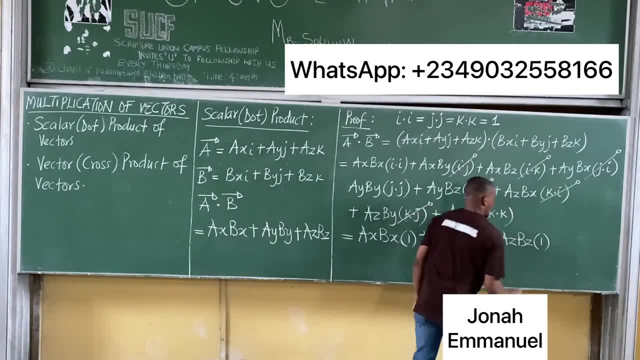 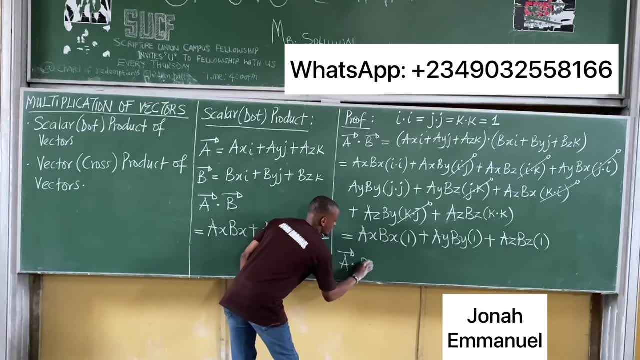 into K dot K. K dot K, we said, is equal to 1. so if I multiply this now, it means that A dot B. so A dot B is now equal to: I have A X B X times 1, which is A X, B, X plus A Y B Y times 1. 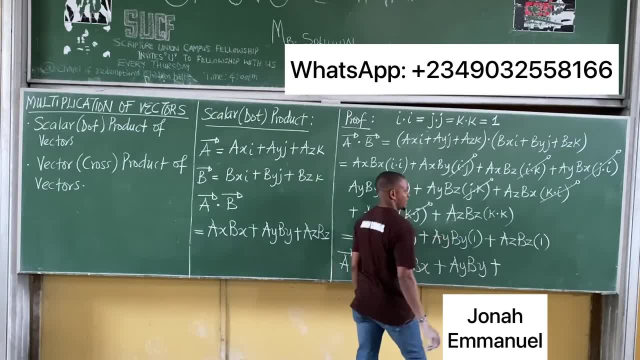 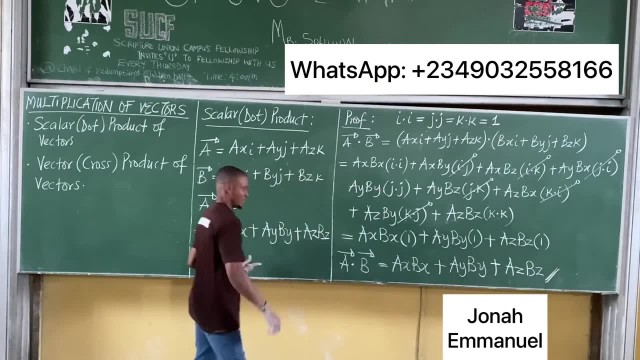 is A Y B Y plus A Y B X times 1 is A Y B X times 1 is A Y B X. so this proves that this formula is correct. this is how we prove this formula. let's look at one more thing and then we can proceed to solving. 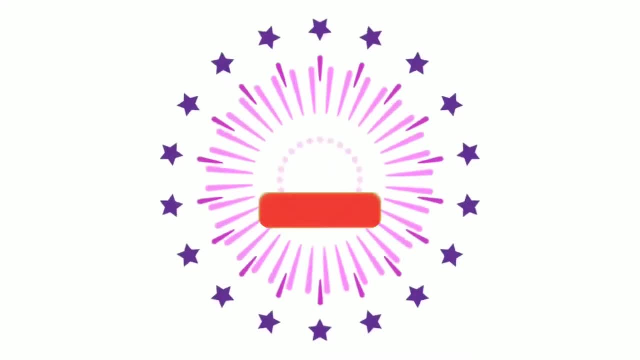 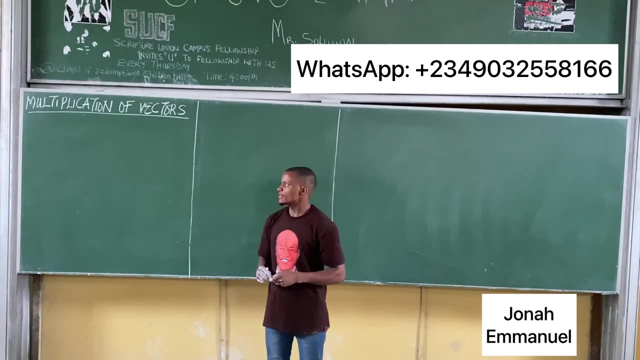 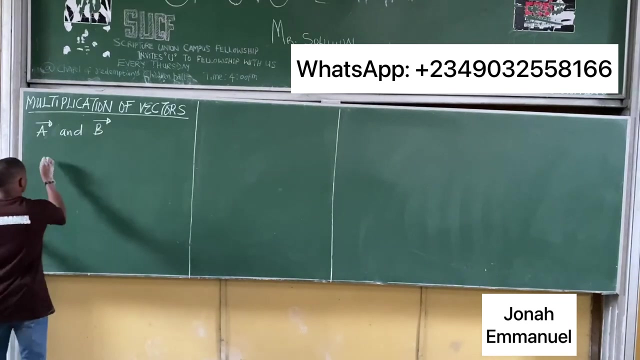 questions. alright, so let's look at um, the dot product of vectors in terms of an angle. alright, given two vectors, A and B, A and B, so vector A and vector B. um, the dot product can also be expressed as: A dot B, B equal to magnitude of vector A. 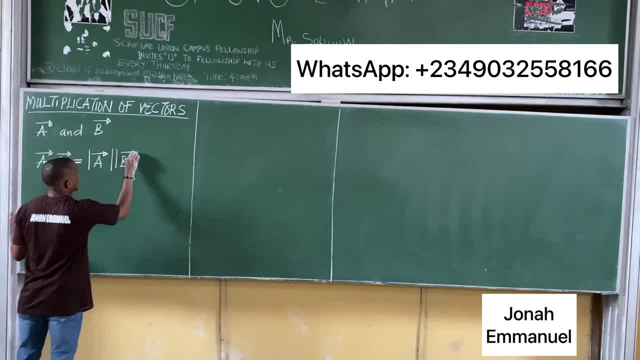 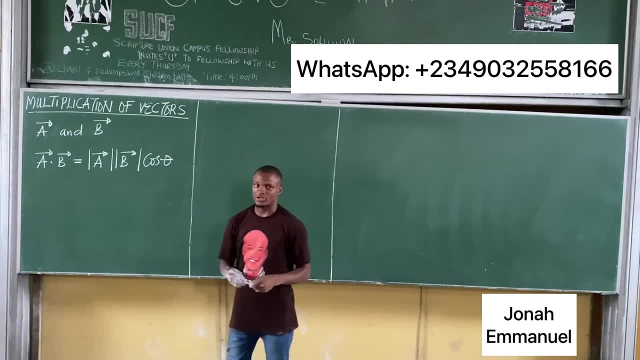 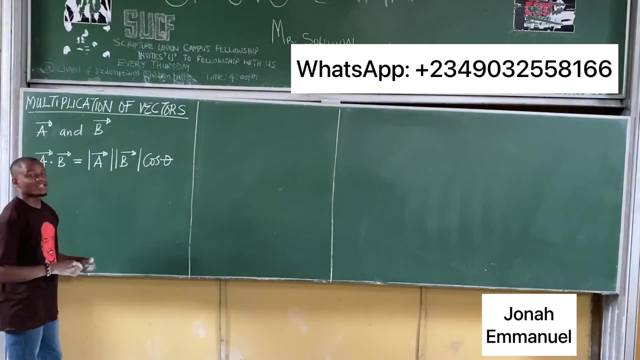 multiplying magnitude of vector B, then cos theta. alright, so this is another expression for dot product. we discussed magnitude in the last class for this one here. this formula can be used to find the angle between two vectors. alright, from here, if I believe, cos theta. subject of the formula. 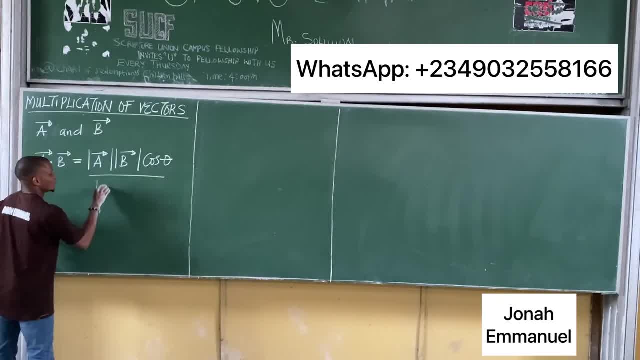 I will just divide this by magnitude of vector A and magnitude of vector B, such that this cancels this, of course. divide the two by magnitude of vector A and magnitude of vector B, so in this cancels this. I have that cos theta is equal to A dot B. 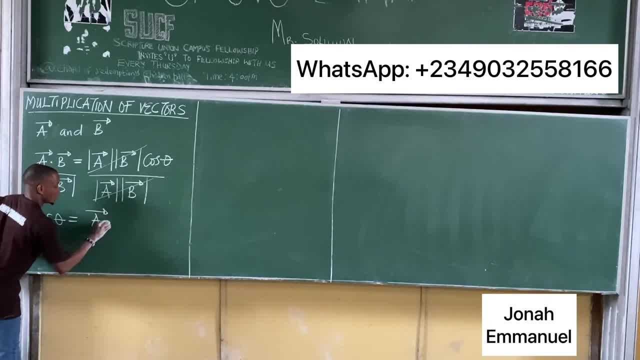 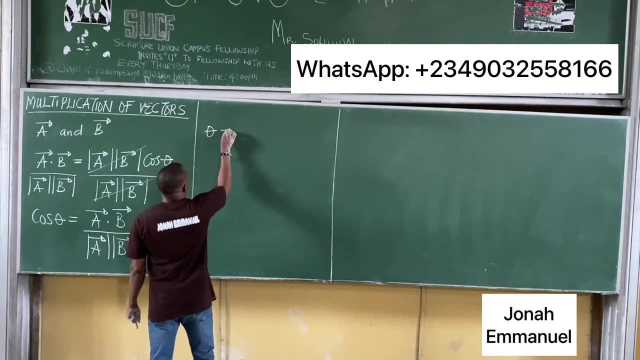 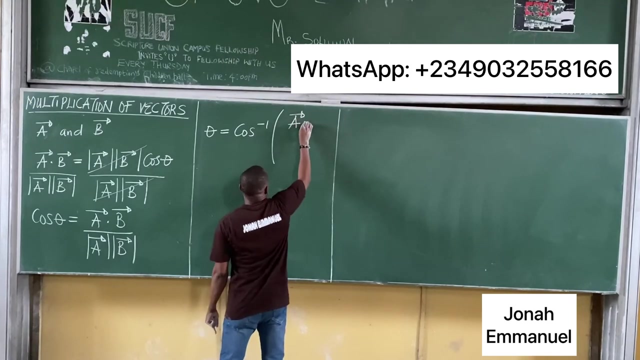 all over magnitude of A dot, magnitude of A dot, magnitude of A dot magnitude of A magnitude of V, such that from here, if I forget theta, theta would be equal to the cosine inverse of A dot B, all over magnitude of A times magnitude of B. so we have: 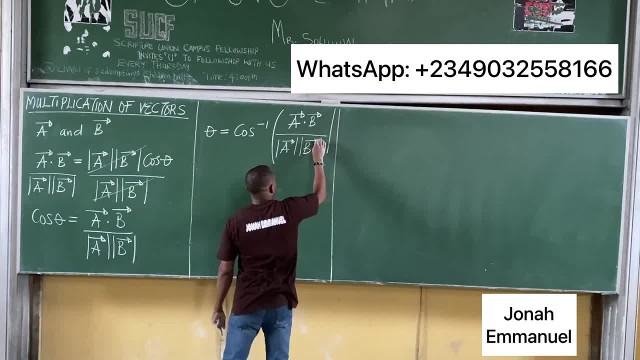 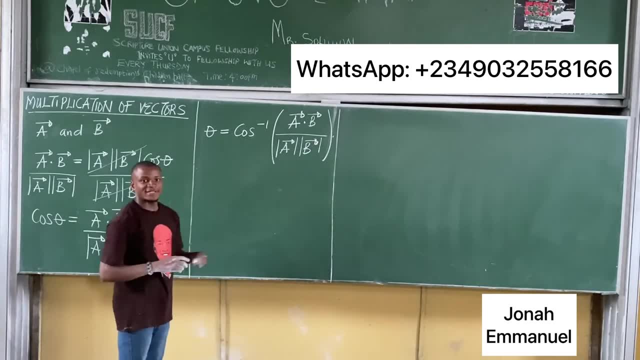 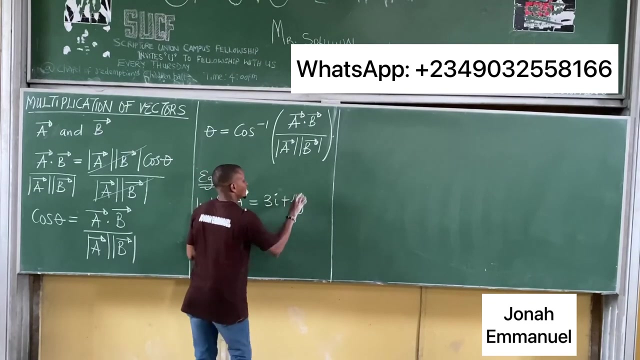 all of this. alright. so we have this. excuse me, we have this and this and this. alright, let's take some sample problems and work them together. so, example example number one: if A is equal to 3I plus 4J minus K and B is equal to, 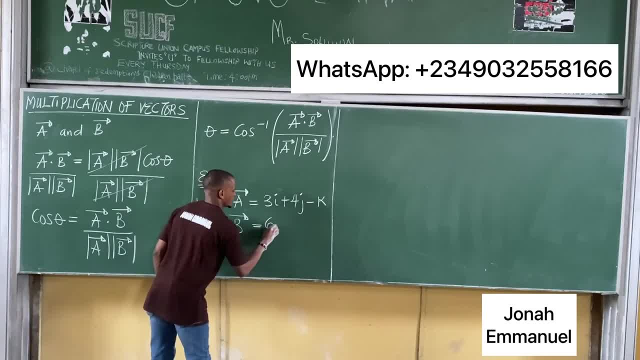 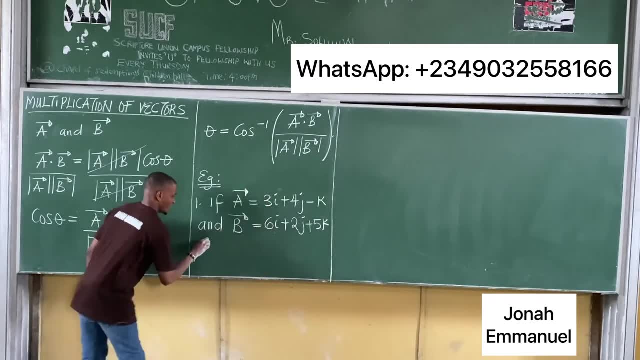 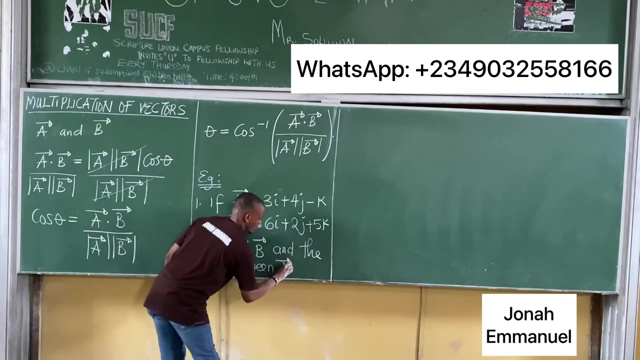 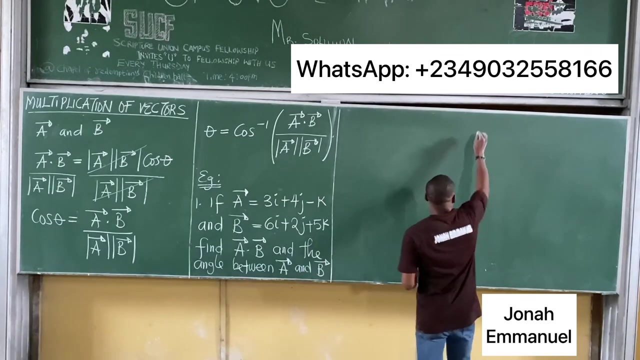 6I plus 2J plus 3I plus 2J plus 5, theta 5 A, dot B and the angle and the angle between vector A and vector B. alright, let's get this so solution. solution to this. first of all, let's get. 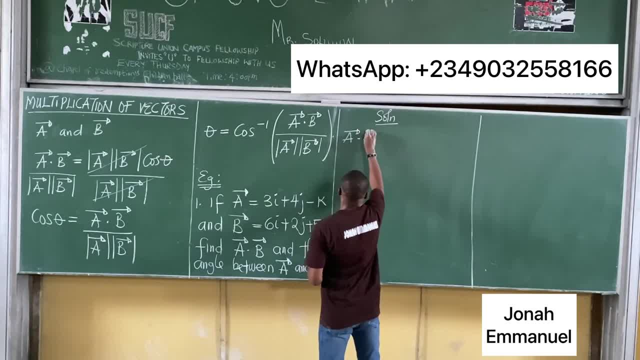 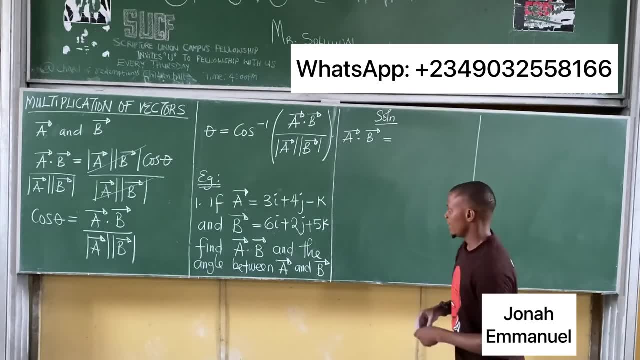 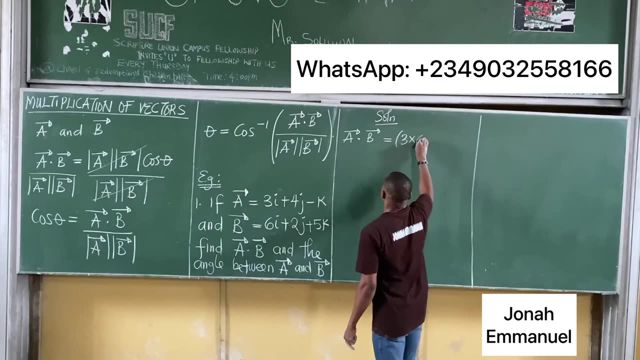 A dot B. so A dot B will be equal to just simply multiply the responding terms like the I's. for I, I have 3 and 6, so it becomes 3 times 6. plus for J- I have 4 and 2 becomes 4 times 2. 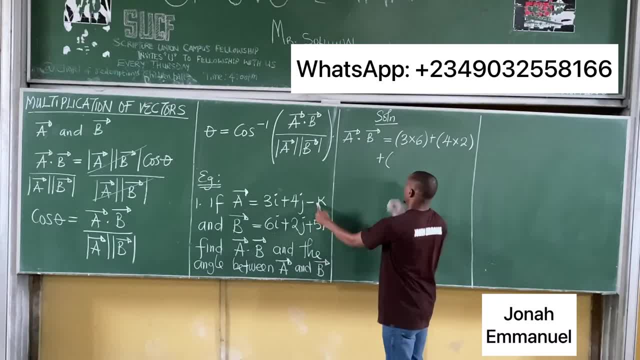 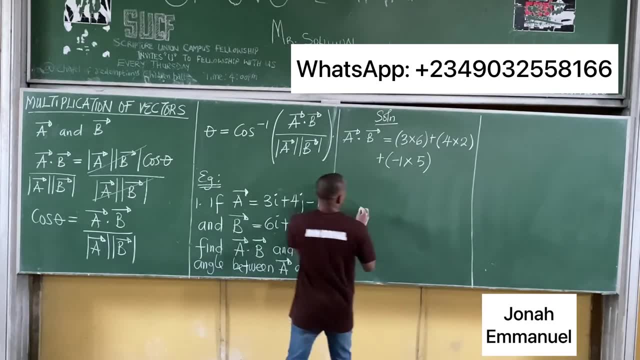 plus. for K I have minus 1 times 5, so minus 1 times 5, so I have this. so that is A dot. B is equal to 3 times 6, is 18 plus 4 times 2, is 8 plus 1. 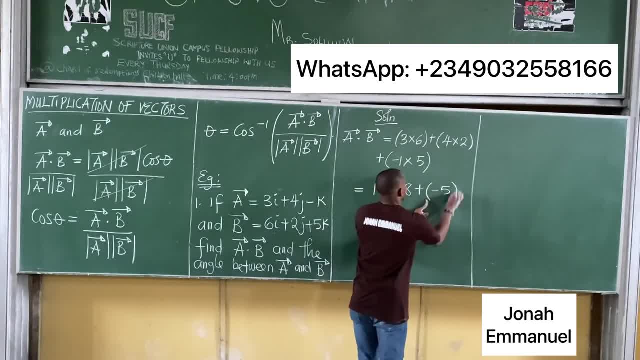 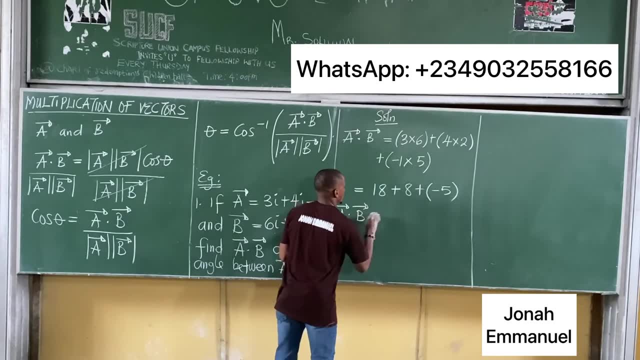 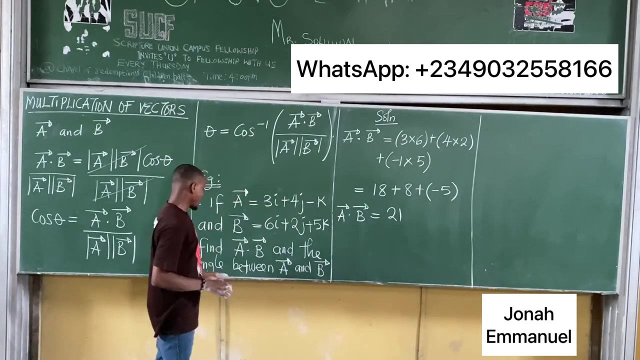 minus 1 times 5 is minus 5. from here it means that A dot B is equal to 18 plus 8 gives 26. 26 minus 5 gives 21. so A dot B is equal to 21. we are asked to find the arm. 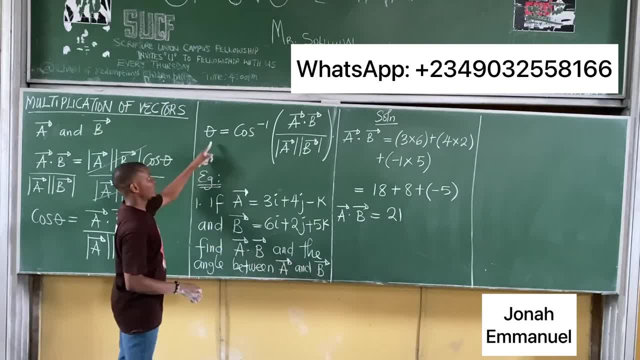 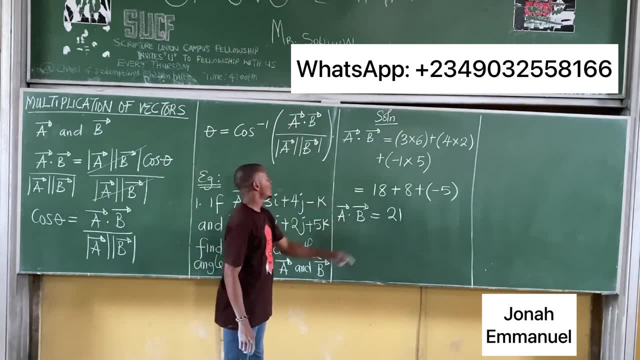 between A and B. to find the arm between A and B is to say that I need 3 A's. I need A dot B, which we've got here. I need magnitude of A. I also need magnitude of B. so let's get magnitude of A to get. 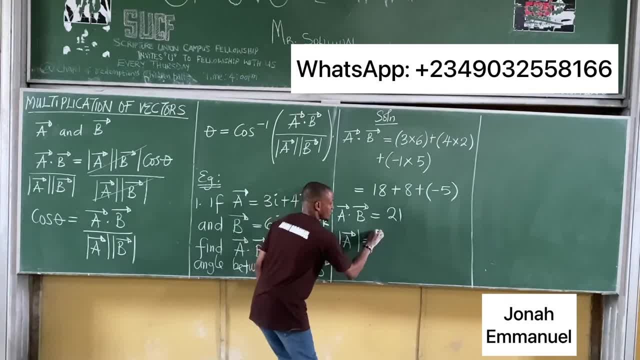 magnitude of A, we said, is simply the square root of each of the 10 square: 3 square plus 4 square plus minus 1, all square. this is equal to. this is equal to: square root of 3 square is 9 plus 4 square. 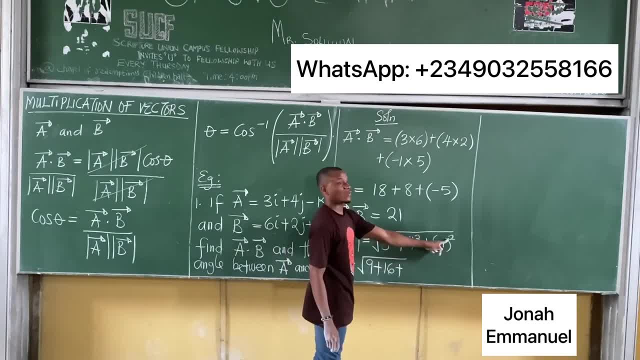 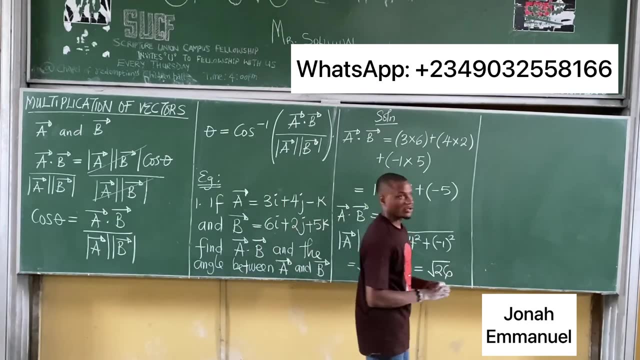 is 16 plus minus 1. all square means minus 1 times minus 1, which is 1. this is equal to 9 over 16, 25 plus 1, 26, so the square root of 26. so that's the magnitude of vector A. 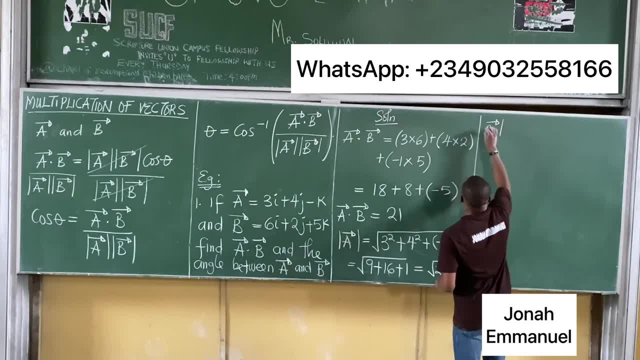 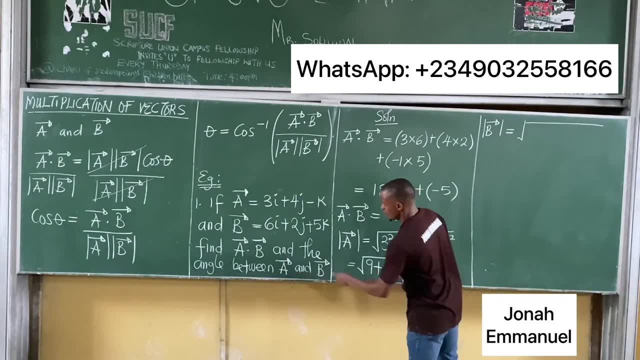 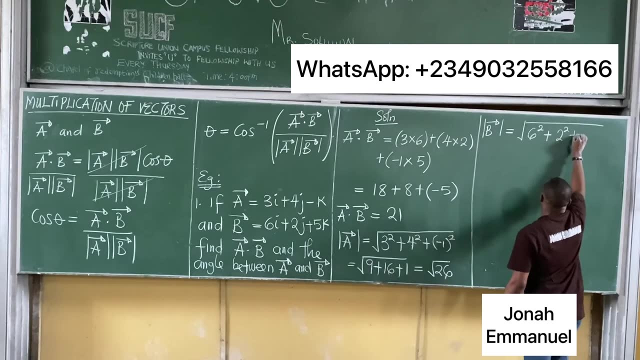 let's get magnitude of vector B- same idea- equal to the square root of each of the 10 square: 6 square plus 2 square plus 5 square. that's equal to the square root of 6 square is 36 plus 2 square is: 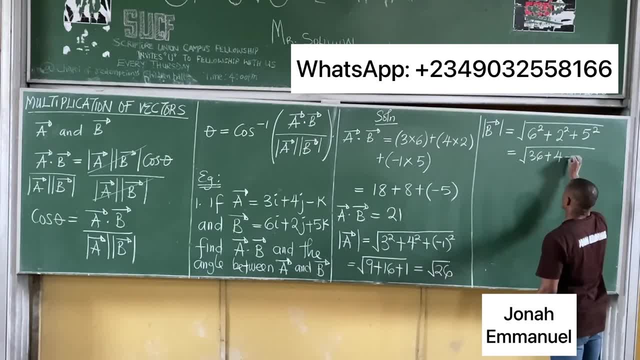 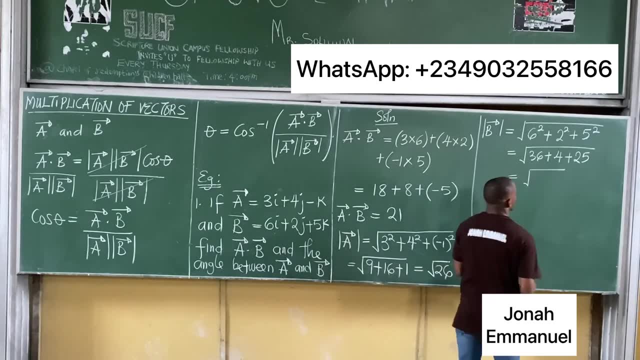 4 plus 5 square is 25 if I sum this up. I'm adding this as being these two here, so this 2 is 29, 29 plus this, that's 5 plus 65, gives you root 65. yes, so therefore theta, the angle between: 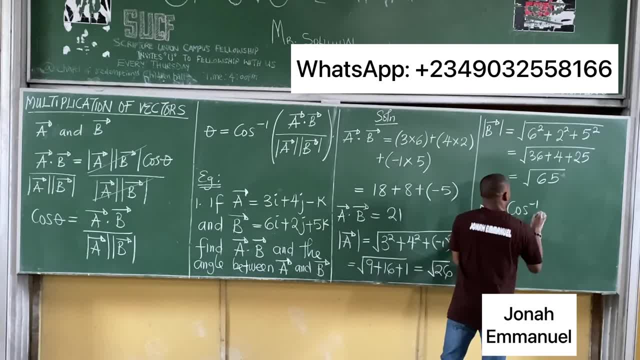 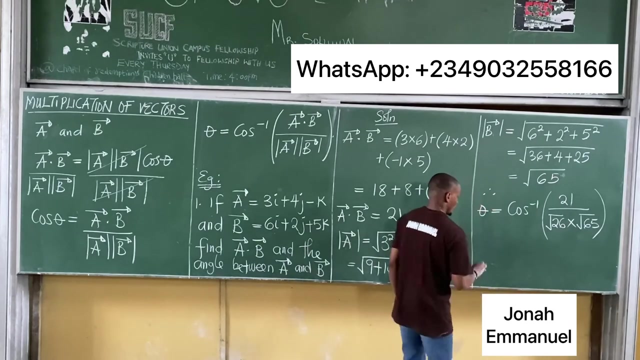 the vector of theta is equal to cross inverse of A, dot A. we said it's 21, so 21 all over magnitude of 26, so root 26 times magnitude of B, which is root 65, so root 65. I harvest 3 harvest, so theta. 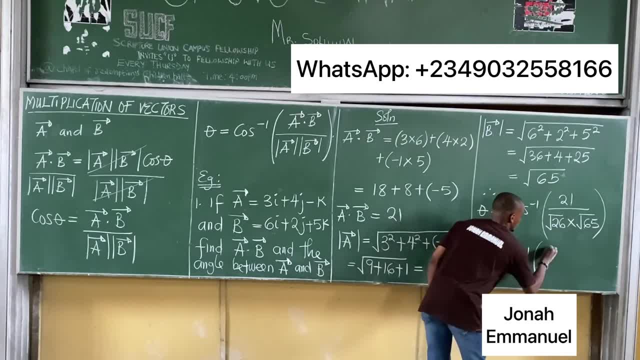 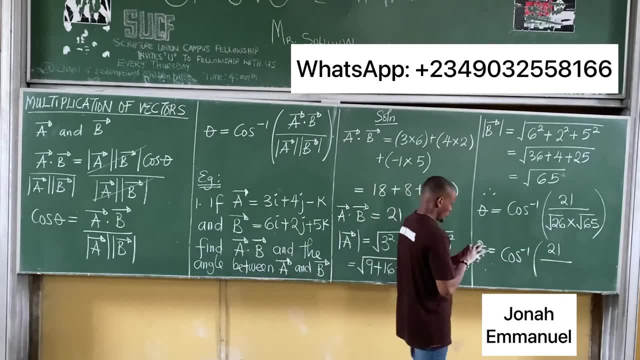 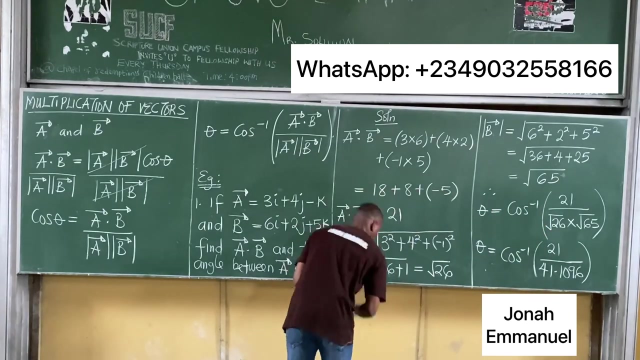 is equal to cross inverse of 21 all over. so I will get the calculator and point this value. so root 26 times root 65, this gives me about 41.1096. so I have this value all right, so get this one here. so that means that 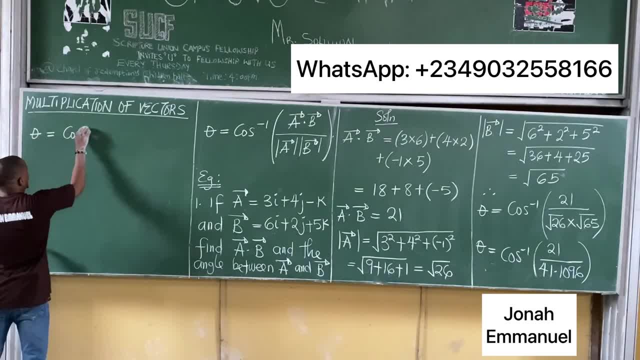 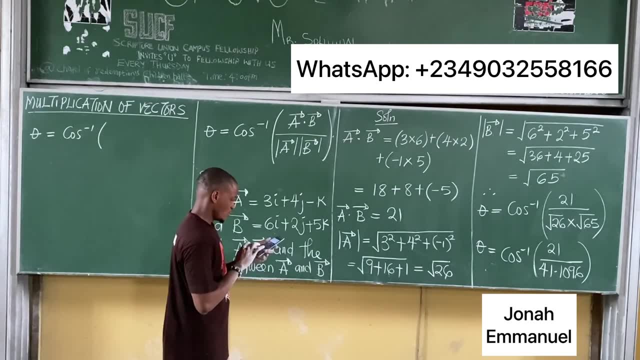 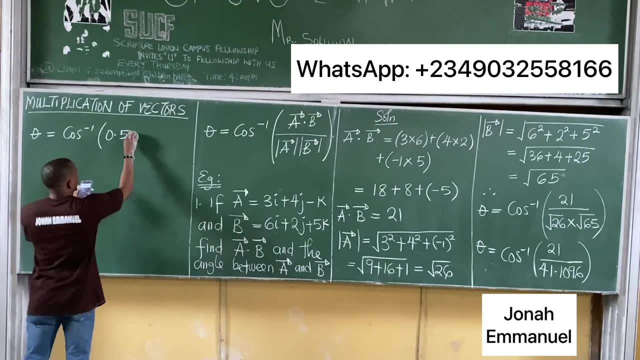 theta is equal to cross inverse of 21, all over 41.1096. all over 41.1096, that gives me 0.5108. so therefore, theta is equal to guess cross inverse, so cross inverse of 0.5108, that gives me. 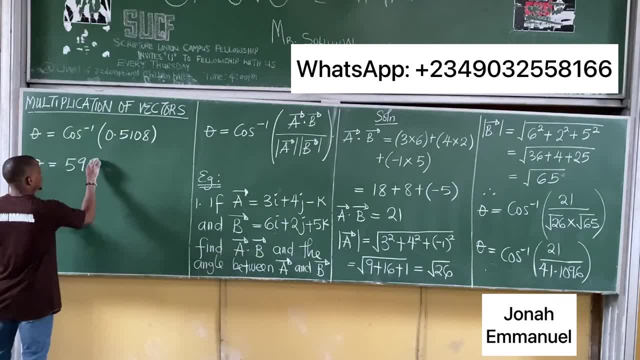 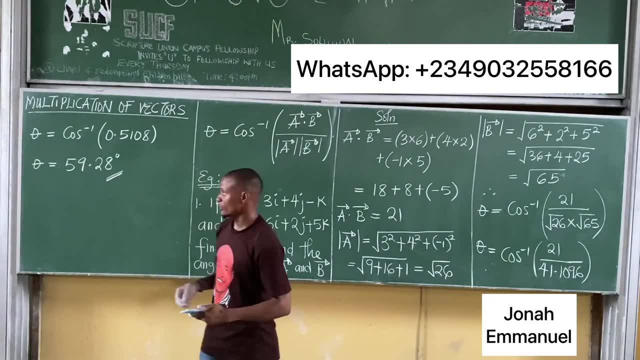 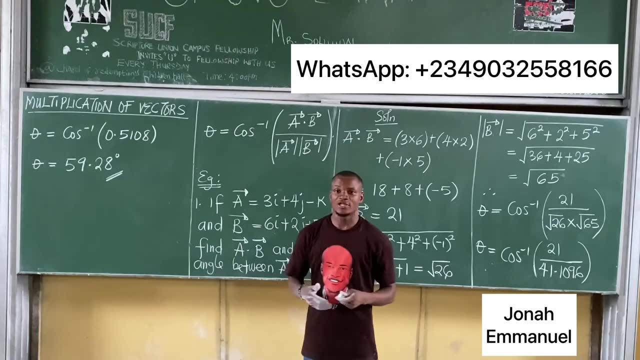 about 59.28 degrees. so this becomes the angle between the vector a and b. so that's how you solve this question. so one last thing on this. you should notice this: if two vectors are perpendicular, it means that the angle between them is 90 degrees.